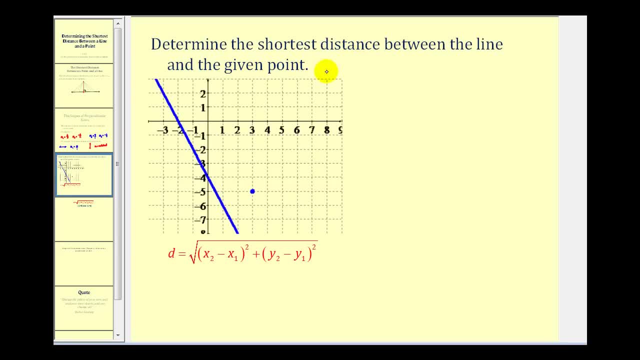 Here we want to determine the shortest distance between the line and the given point. The given point has coordinates three negative five. So that's going to be one endpoint of the segment. And then the question is, what is the other endpoint of the segment that's perpendicular to the given line? So our first step would be to determine the. 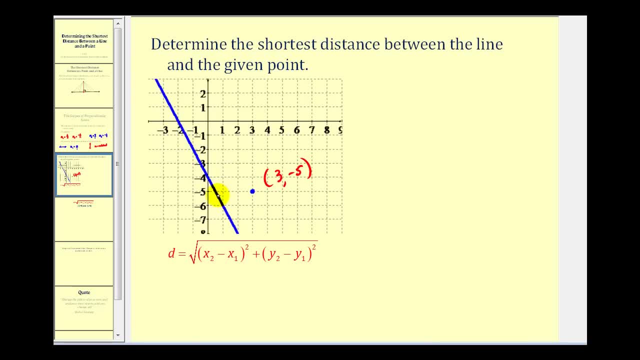 slope of the given line. So let's go ahead and pick two convenient points. Let's say this point here and this point here. I say convenient because the coordinates of these two points would be integers, And now we can make a triangle to represent. 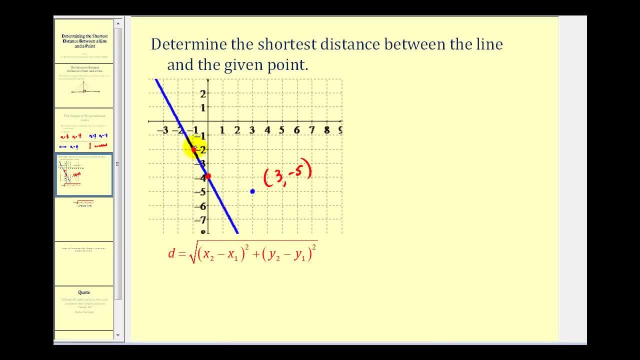 the change in y with respect to the change of x. So to go from this point to this point, notice- we have to go down two units, So that would be a negative two, and then we go right one unit. This tells us the slope of. 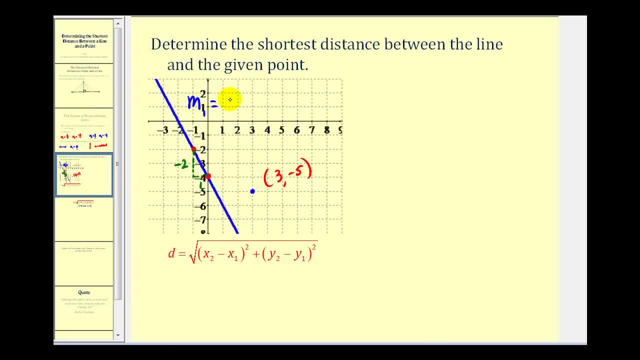 this point of this blue line is equal to negative two over one or negative two. Now, the reason that's so helpful is the slope of the segment here that's going to give us the distance between this point and this line would have a slope. that's the negative reciprocal. 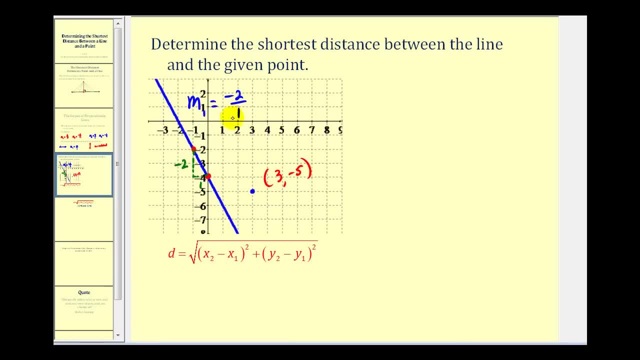 of the blue line. So the slope of this perpendicular segment would have to be the negative reciprocal of negative two over one, which would be positive one over two or one half. So now we're going to go ahead and sketch the line that passes through this point. 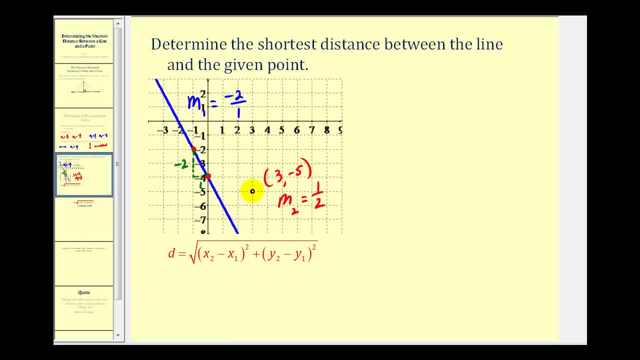 that would be perpendicular to the blue line, And then we can determine the other end point of this segment. So from this point we'll use the slope to find another point on this line. So we'll go up one and right two, And now we can go ahead and sketch the line that's perpendicular. 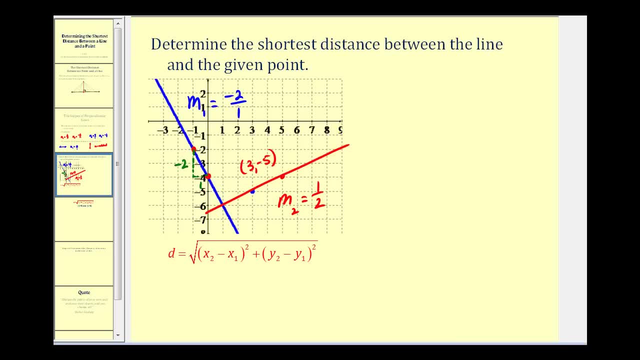 to the blue line. Now, even though we just sketched the line, remember we're only concerned about the coordinates of the blue line. So the segment with one end point here at three negative five and one end point here at the intersection. 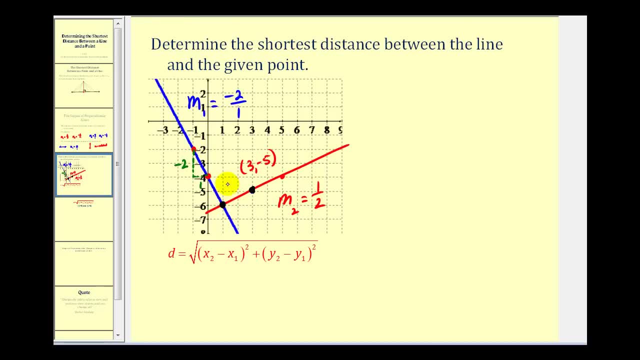 of the red line and the blue line. So the coordinates of this other end point is going to be one negative six. So now we'll find the distance from one negative six to three negative five, And this will be the shortest distance from.